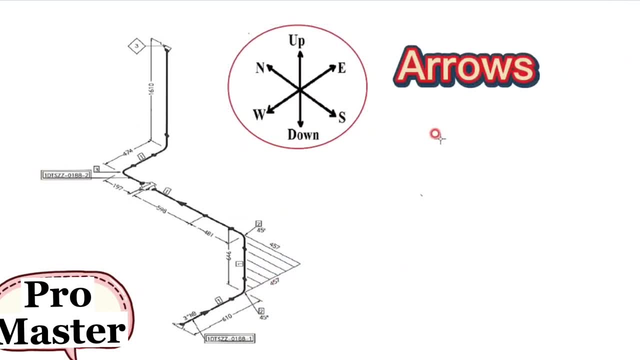 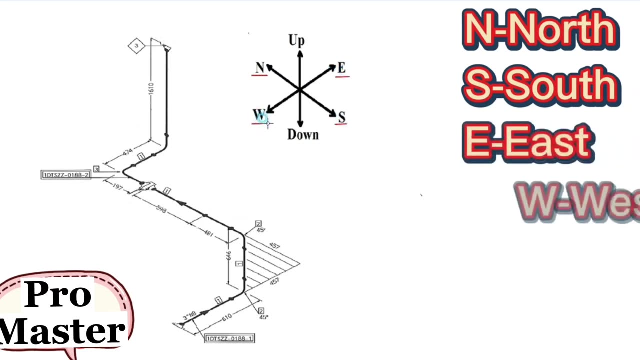 There are six directions here. By studying these directions we can easily read the pipe isometry. We will start reading the pipe isometric from this point, because the direction of the pipe isometric is the direction of the pipe isometric. The direction of the arrow on the pipe drawing is in this direction. 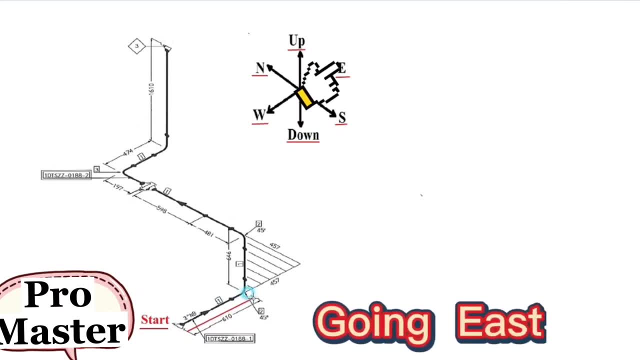 The pipe travels start from this point to the east direction. There is angle of 45 degrees. Therefore the pipe travels to the east, then it travels north direction at an angle of 45 degrees. Then the pipe travel continue to the north direction. 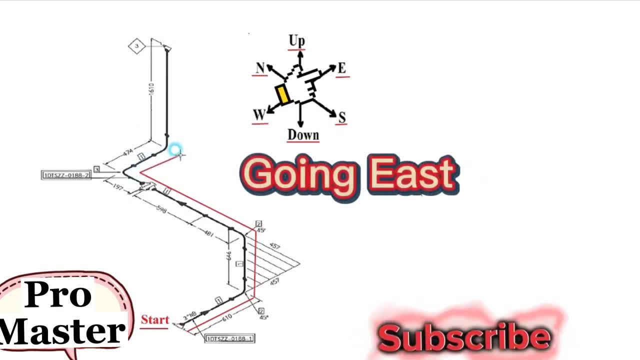 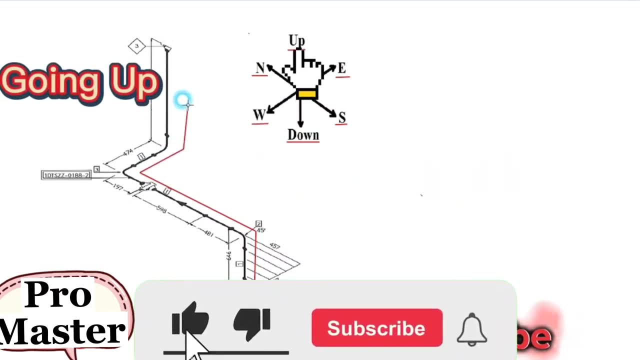 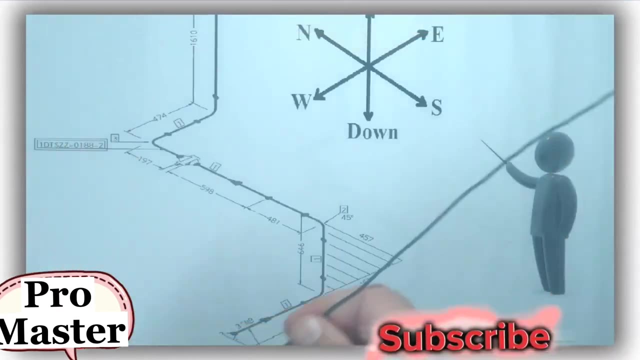 In this point the pipe travels to the east direction. Then we pipe travels continue to the up direction and the correct reading of the pipe drawing is completed. Now let's bend the wire of this pipe drawing. This is our wire, the sketch showing these directions, this is the pipe isometric. 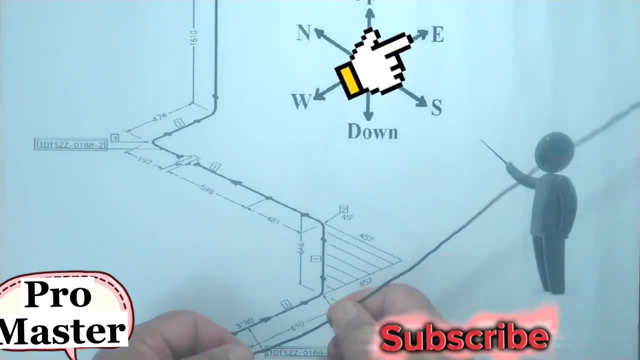 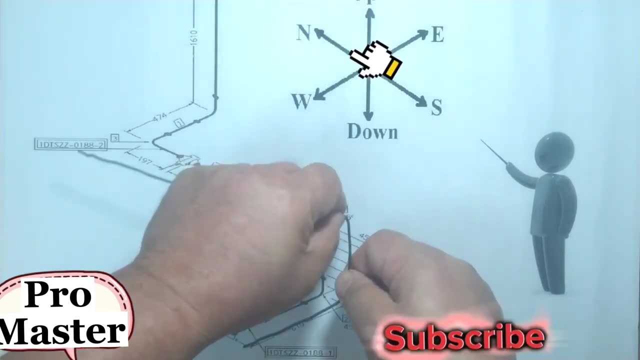 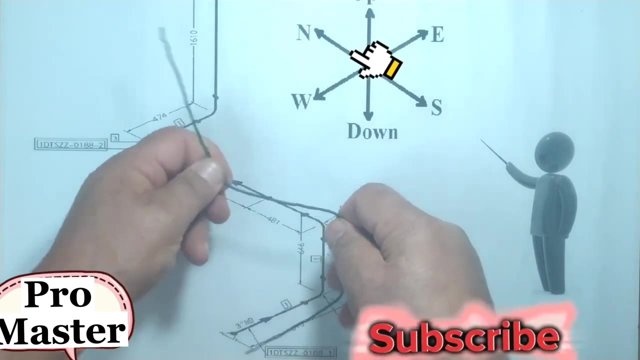 Since the pipeline is traveling to the east direction, we hold the wire in the east direction, Then the wire bending first to the east direction, then to the north direction by 45 degrees. Then the wire continues to the north direction. It is under 40 degrees and the wire is moved by the power of strong current. 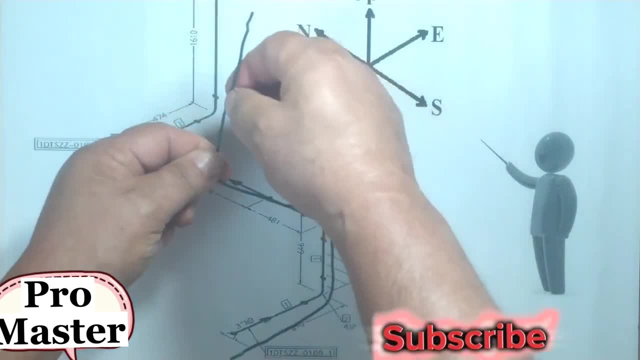 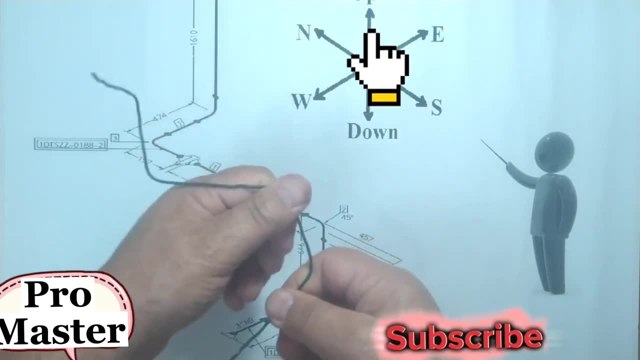 Since it is in the north direction, we hold the wire last. then we bend it to the east direction. The которое, which is the direction of the pipe, isometric. at this point it circles to the outtorking. We bend the wire Link this point to the north. 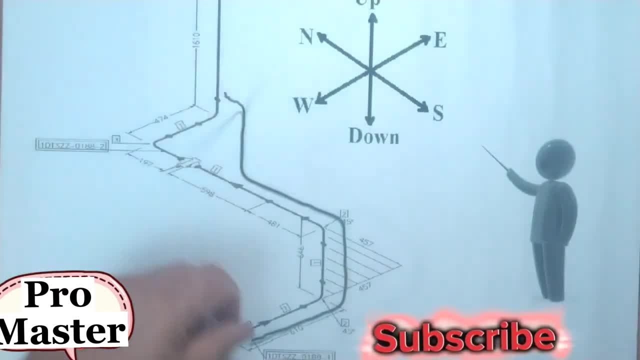 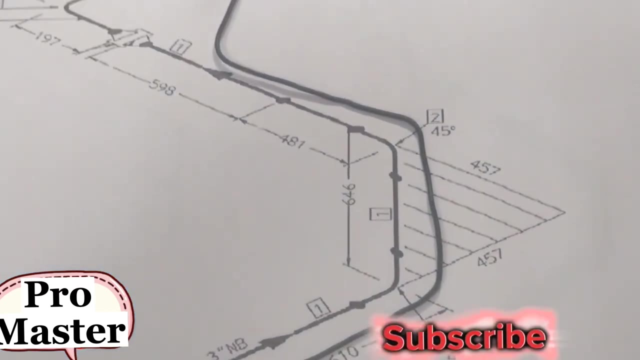 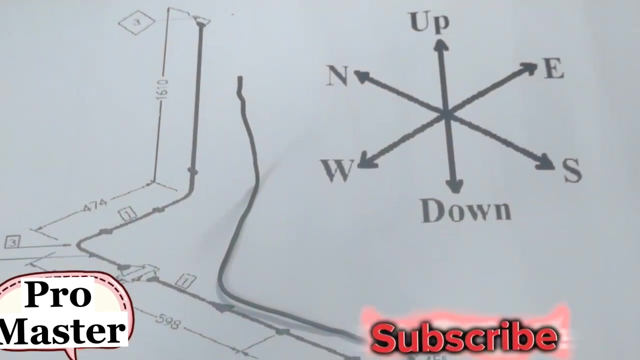 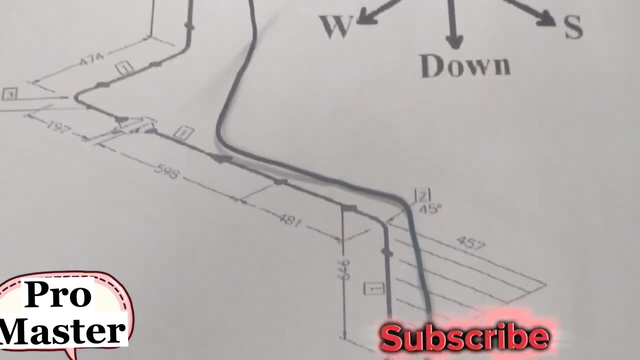 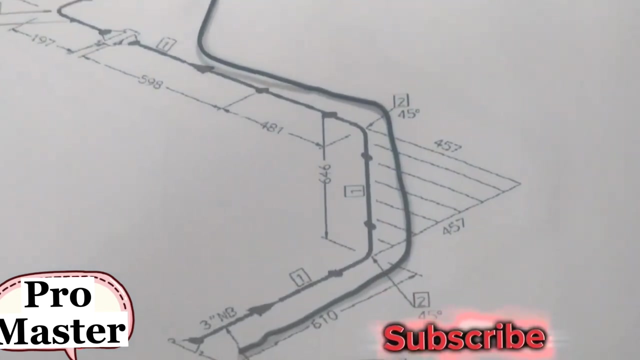 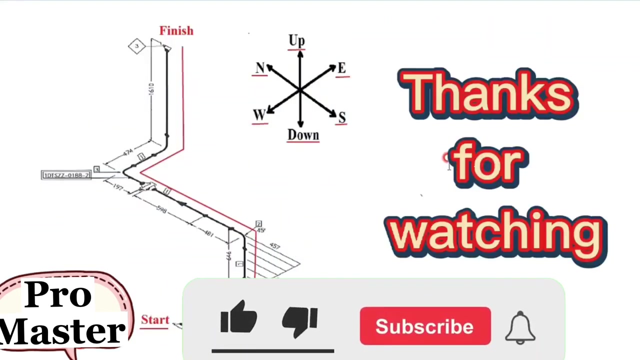 Thank you. Subscribe to our channel. Thank you for watching.